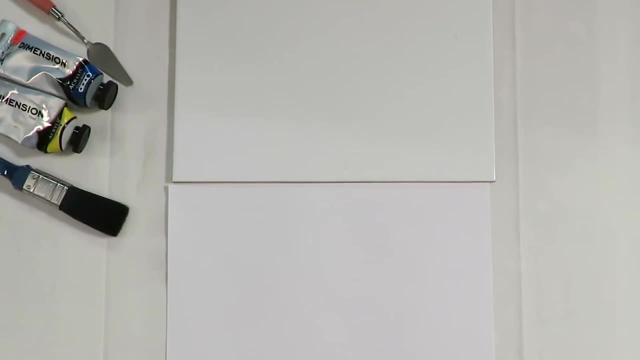 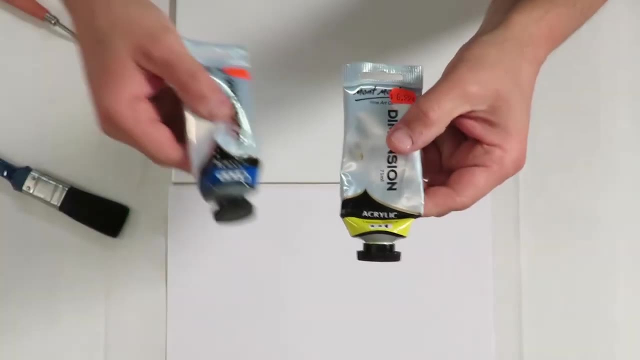 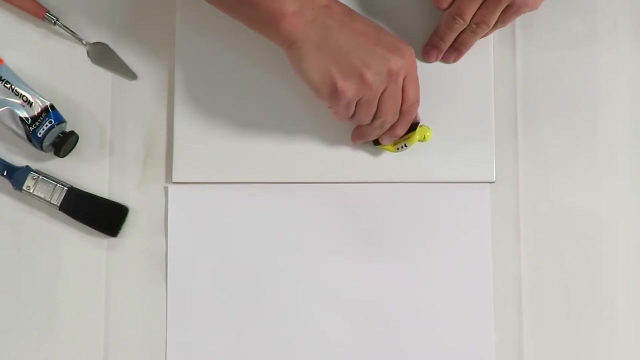 G'day everyone. in today's video I'm going to show you how to make chartreuse paint color. I'm using lemon, yellow and cyan blue. Okay, put some yellow paint here and just a small amount of blue. Okay, now we just get the tiny little bit. 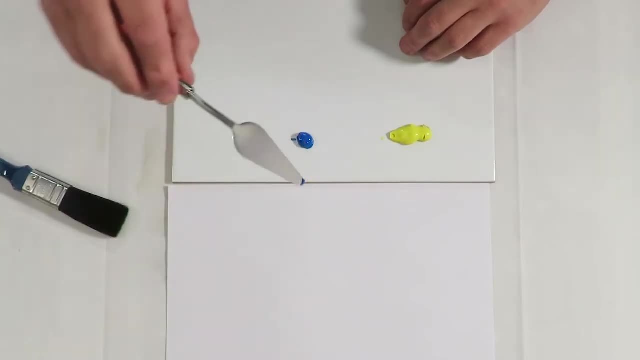 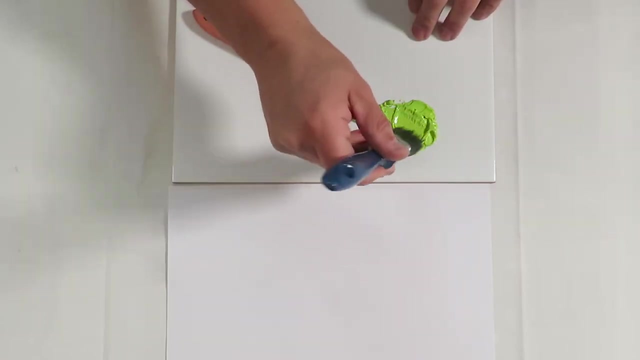 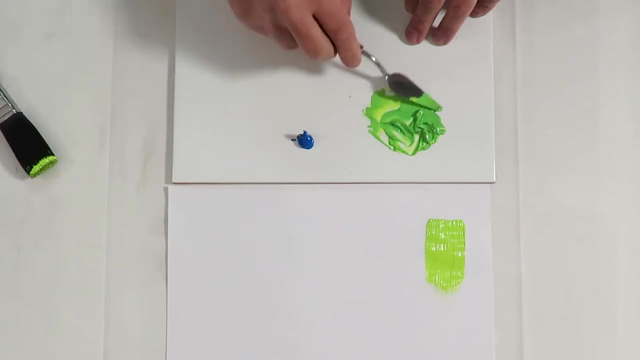 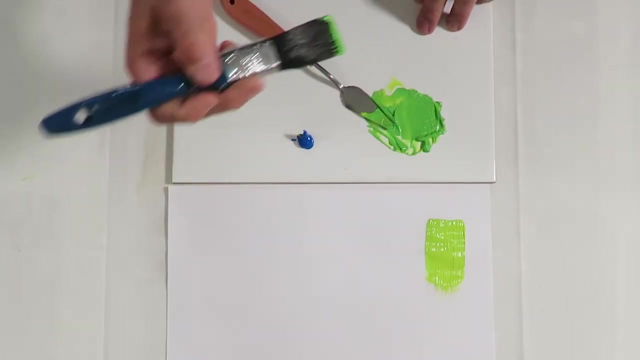 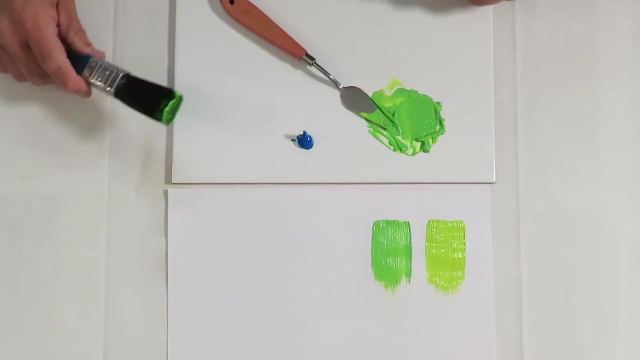 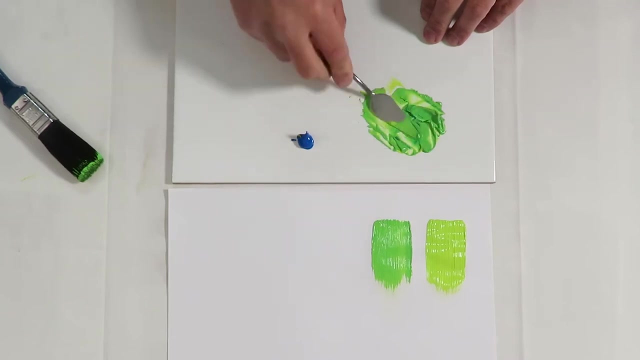 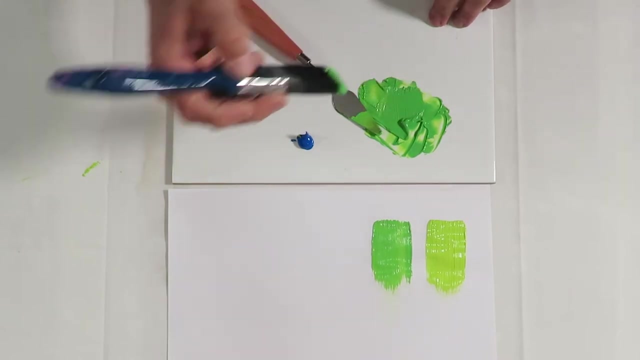 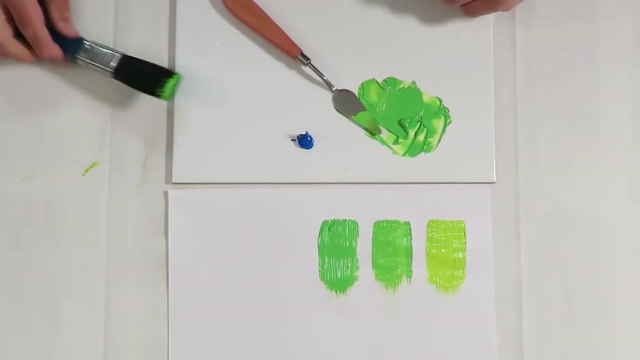 of blue on the palette knife, Just a little tiny bit like that, and mix it up in the yellow, Mix up to more blue and change the color a bit more. As you can see, you don't need much blue, Oh boy. Now I'm going to do the same thing with the other side. 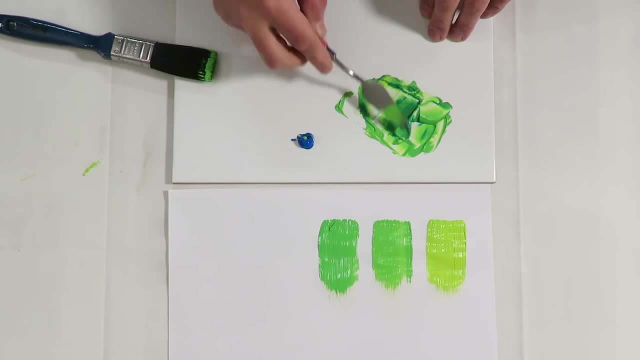